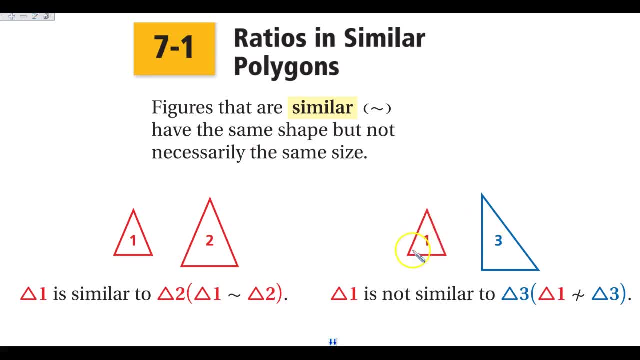 If we look over here at 1 and 3, okay, this triangle 1 was the same as this triangle 1, but notice that this looks like it's isosceles. and then this is right. These are not the same. 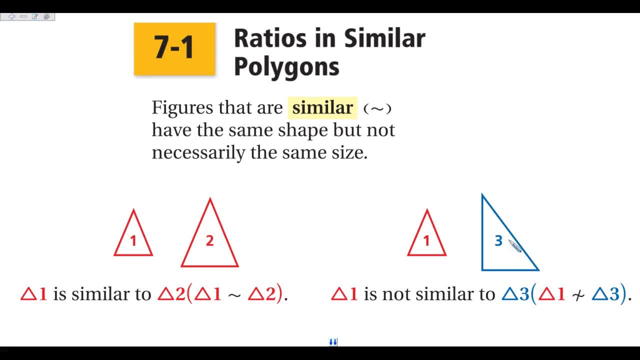 type of triangle. They are not the same shape- triangle, So they're both not the same shape. and they're not the same shape- different sizes, so they are not similar, All right, so one thing that I want you to notice is the symbol that we use for similar is right here. that is a tilde. Okay, so I can say that triangle one. 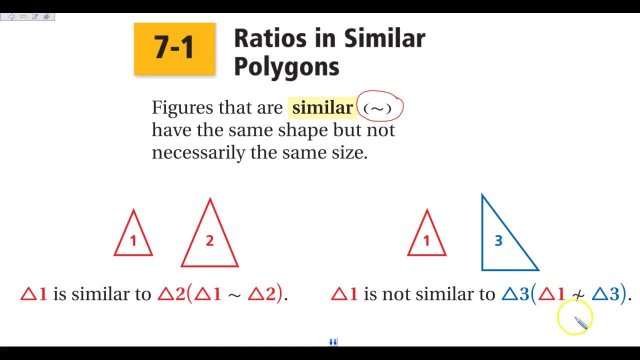 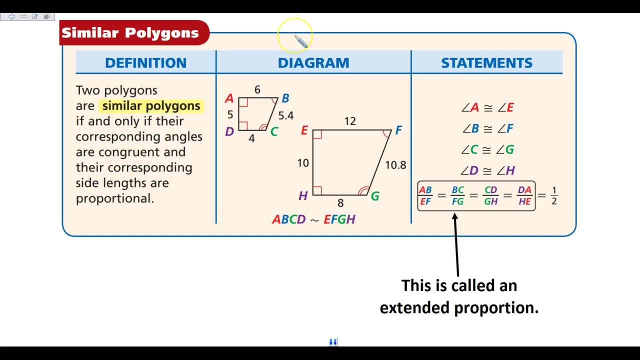 is similar to triangle two, Okay, or I can put a slash through it for not similar, All right. so if there's any questions about that, make sure you are making notes on your paper and we will get those answered. But let's take a look at a look a little more at what similarity means, Okay. so if 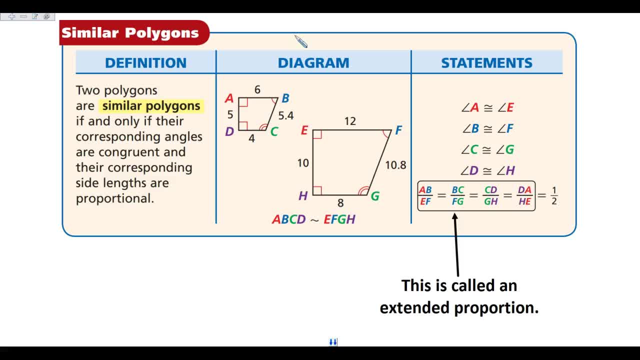 I have two figures that are similar. Okay, their corresponding angles are congruent. Their corresponding sides are proportional. So let's think back for a second, when we did congruent triangles and we said that when we knew that our triangles were congruent or congruent figures. 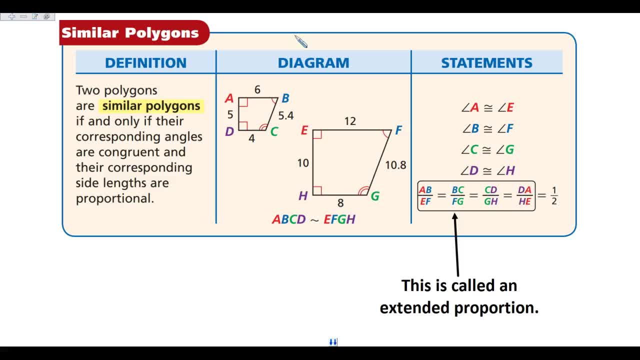 we had, or if we had, congruent figures, we knew that all the pairs of angles were congruent, All those matching angles. That doesn't change with similarity. So if I look here, angle A and E are corresponding Angles and they're both right angles here, So they are congruent. Angle D and H: same thing. They. 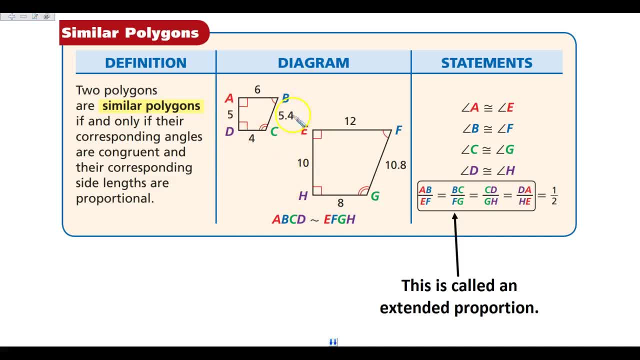 are both going to correspond and they are congruent. If I look here, B is going to correspond with F- They are congruent- and angle C is going to correspond with angle G, So they are congruent as well. So if we look over here, all my pairs of corresponding angles are still congruent. Now 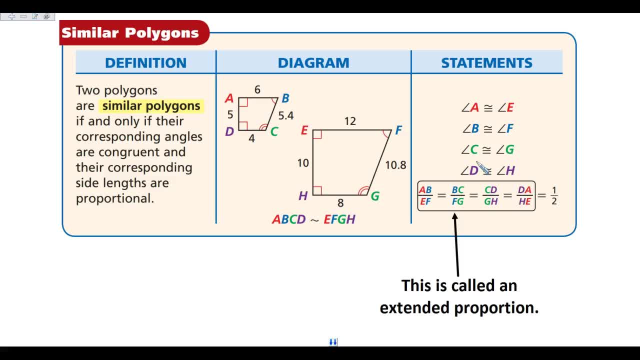 with congruent figures, our corresponding sides were also congruent. We're going to change that up a little bit here with similarity and we're going to say that our corresponding sides are proportional. So what that means is that if I take the sides in one figure, 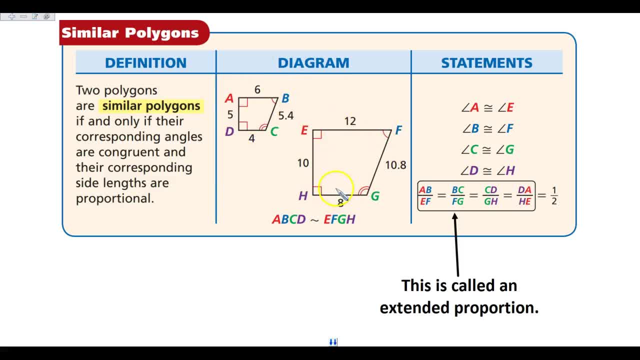 and I put them over the sides in the other figure, they will all reduce to the same fraction. So if I look at AB over EF, that is 6 over 12, which is going to reduce to one half. So I'm doing little figure over big figure, Okay. 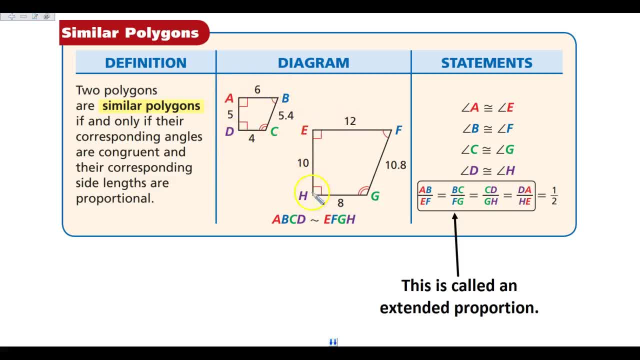 So 6 over 12 is one half. If I look here at AD and EH, that is 5 over 10, which is also one half. CD and GH is 4 over 8, which is also one half, And BC over FG is 5.4 over 10.8, which is also one half. 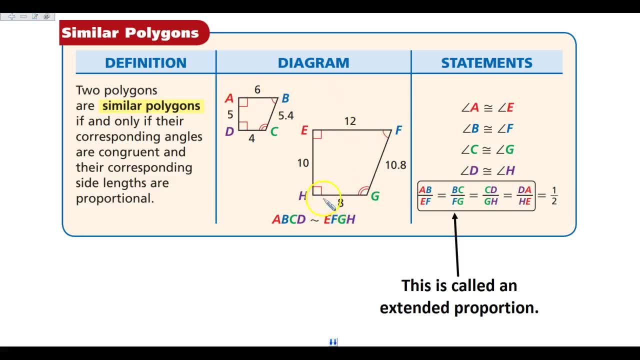 So each side length is a different length, but when I put my small side over its matching big side, they will all reduce to the exact same fraction. That's what it means to be proportional. So when I look over here, I have that fraction that AB over. 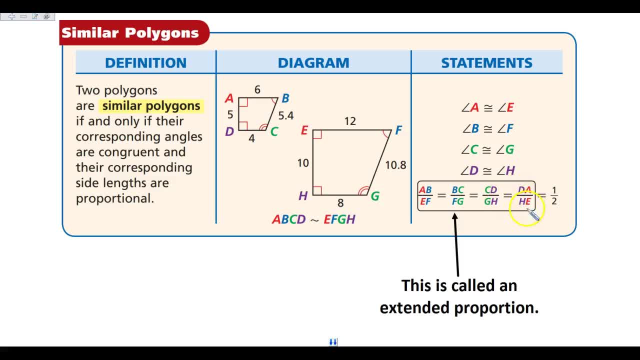 EF, BC over FG, CD over GH, DA over HE. All of those fractions equaled one half. So what this is called here, with all of my side ratios, is an extended proportion. When I'm writing, all the sides are, their ratios are equal. Okay. 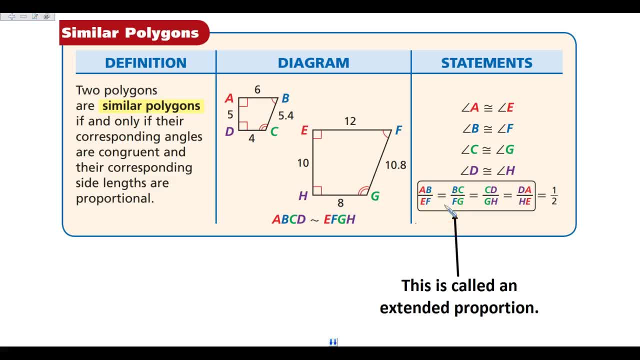 Remember AB over EF. AB over EF is a ratio. Okay. So when I'm looking here, my extended proportion has in the numerator: all of these are the small figure In the denominator. this is all the larger figure. Now, it does not have to be small over large. It could be large over small. and then my similarity. 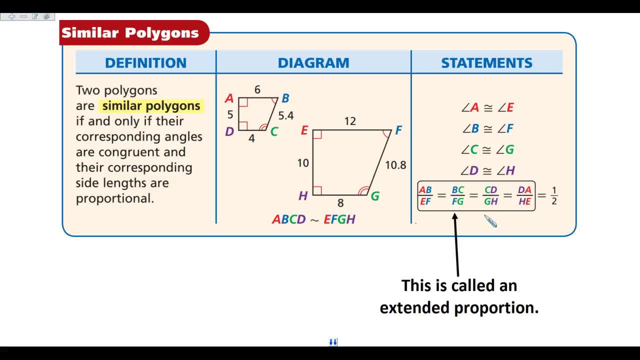 ratio would have been two over one. But it's the important thing here is that I have the same figure in the top, the other figure in the bottom. You cannot mix and match those. It's very important that you keep a consistent figure in the numerator, a consistent figure in the denominator. 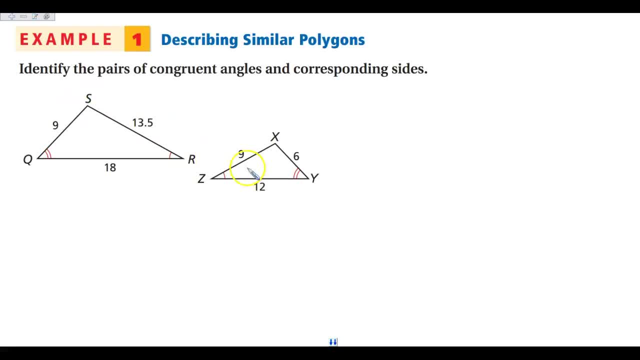 All right. So let's take a look. We're looking at these two triangles here and I want to identify all of my pairs of congruent angles and all of my corresponding sides. So what I'm going to start with is looking at my corresponding sides, But sometimes with the 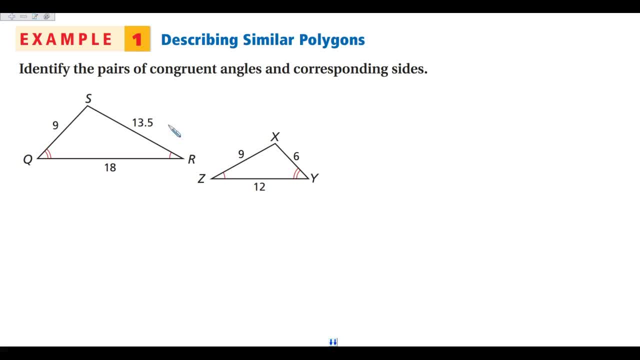 similar figures, it can be a little difficult to see what matches up with where, because they are different sizes. So what I'm going to do is, when I'm looking at my sides, I'm going to find my smallest side. If I'm looking at this figure here at triangle QRS nine is the smallest side length. 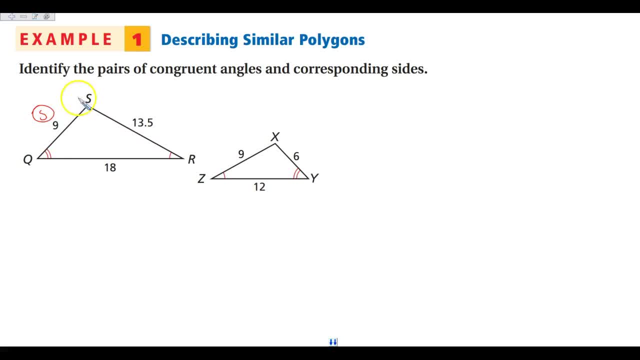 Okay, So I'm going to label that as S for my small side, My 13.5. here is the next biggest side. So I'm going to label that as M for my medium length side. And then QR- here is 18. So I'm going to label that as L for the longest side. Then I'm going 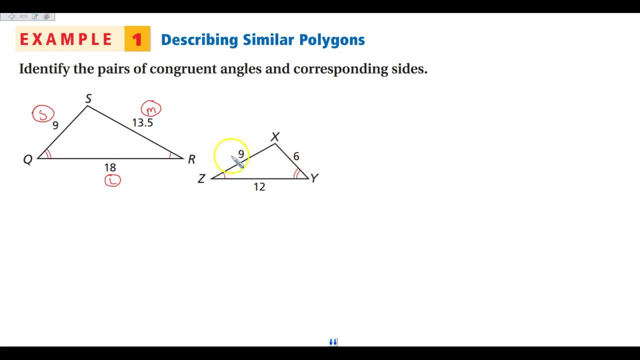 to come over here and do the same thing. So over here in this triangle XYZ, six is my smallest side, Okay, Nine is the middle side and 12 is the longest side. So doing this allows me to match up my small sides easier. So my smallest side over here is QS. 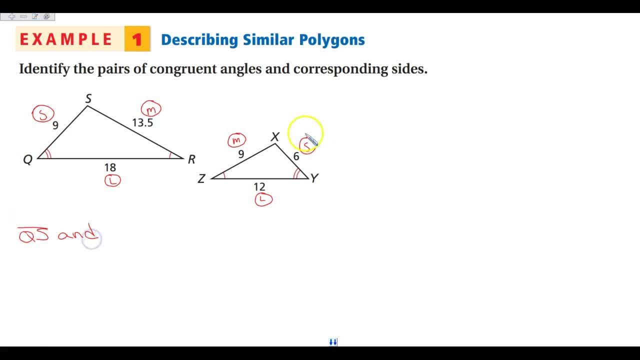 So QS and my smallest side over here, which is XY, those are going to be corresponding sides. Okay, Then I'm going to do the same thing with my medium length sides. SR is my medium length side over here, So it'll be SR and my medium side over here is XZ. 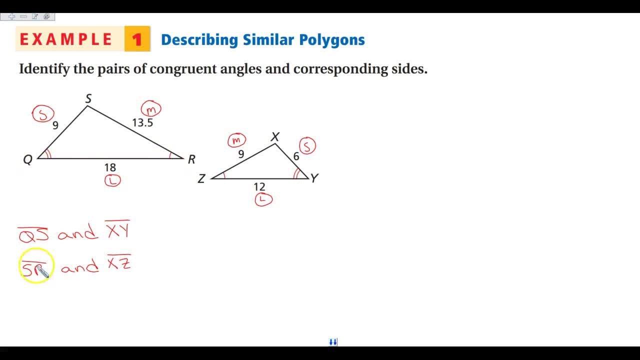 And then I'm going to take a look at my longest sides, which in the first figure is QR, which is 18.. So I'm going to take my longest side over here and my medium length side over here is QS. And then I'm going to take my longest side over here and my medium length side over here is YZ. 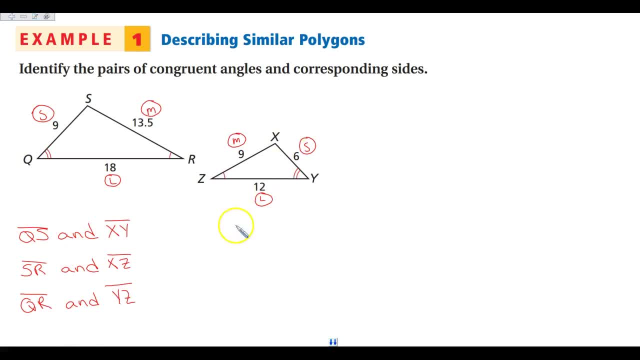 So those are all of my corresponding sides by using their side lengths to help me match them up. Okay, Then we're going to look at our corresponding angles. My- here, my one arcs are going to be R and Z. So angle R is going to be congruent to angle Z Because, again, in your similar figures, your angle 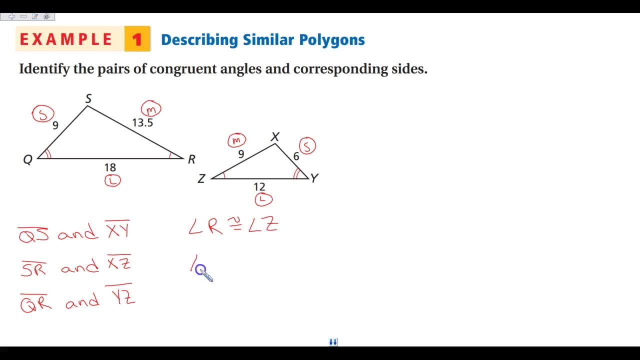 measures are still congruent. All right, My double arc here is Q. My double arc here is R. Okay, here is y. So angle q will be congruent to angle y, And then my one without any arcs, is s and x. 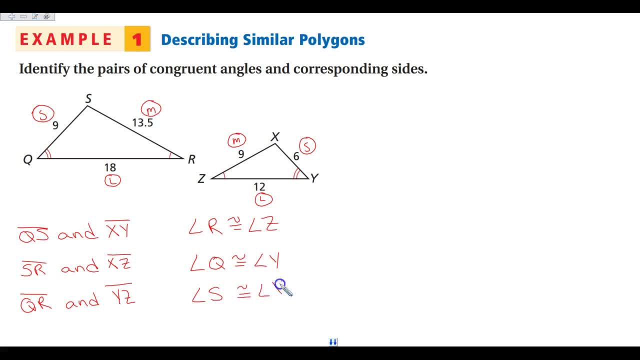 So angle s is congruent to angle x. And again, we know that these are congruent because we can use our third angle theorem if we need to, Because remember, in a triangle, if you know two pairs are congruent, then the third pair must also be congruent. Okay, so that's our third angle theorem. 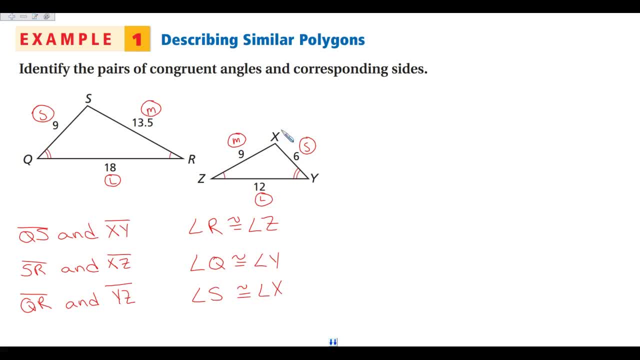 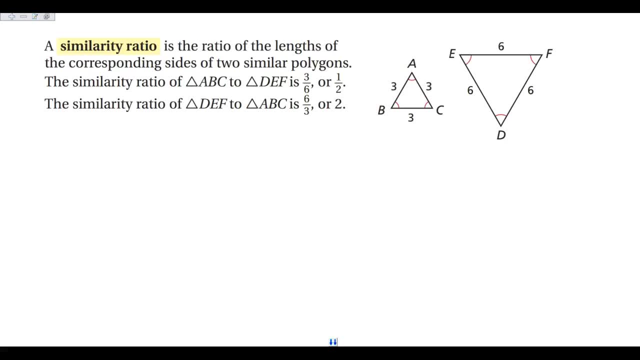 but they're going to correspond as well, All right. so if you have any questions on that, please make note of it. All right, we are going to look right now at what a similarity ratio is. Okay. a similarity ratio is the lengths of the corresponding sides of our polygon. So if we come 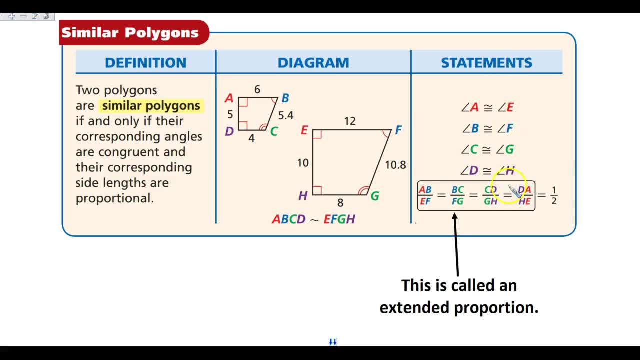 back here, to this first slide, for our second slide, for a second. remember when, we did you know, six over 12 was one half. five over 10 is one half. four over eight is one half. Well, the similarity ratio of my small figure to my big figure is one half. 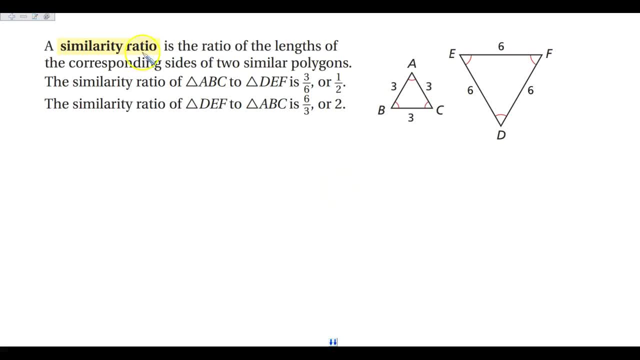 So when we're doing this, we're going to look at the same thing. Okay, so if I'm looking here at abc2def, remember that this word two tells you the order in which you're supposed to look at your figures. So that means that abc is going to go in my numerator and def is going to be in my. 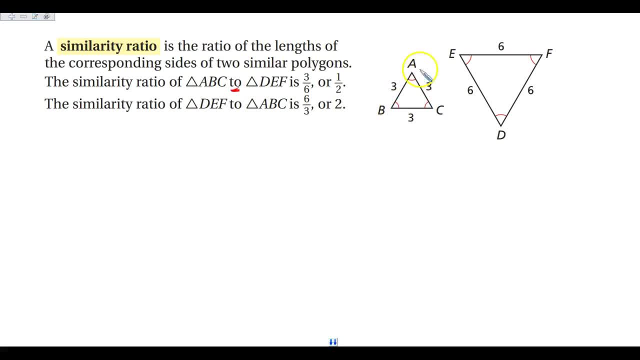 denominator. Okay, so abc is all my sides are three, def all my sides are six. So I'm going to do three over six, which is one half. Now if I do my similarity ratio the other way of my big triangle to my little triangle. 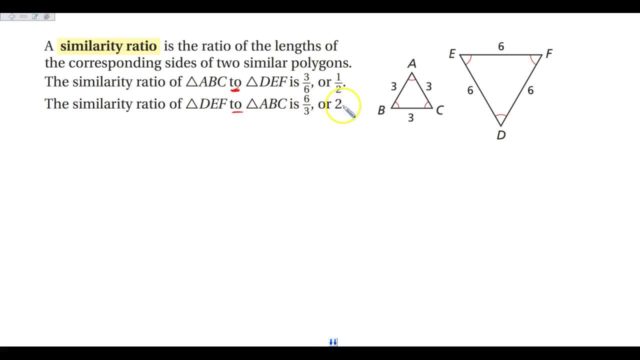 it'll be six over three or two, And you can also say two to one, if we're looking at that. Okay, remember, we can write a ratio as one half, we can write a ratio as one to two, or we can say one- two. 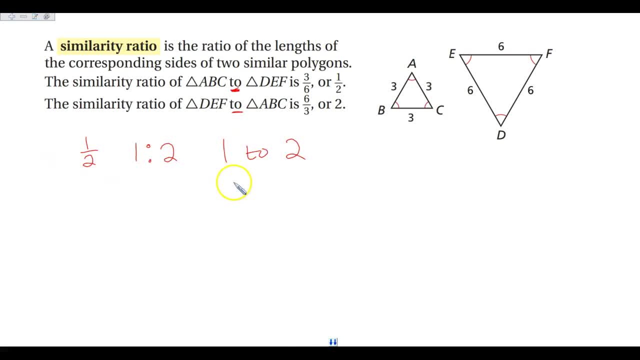 two, All right. all three of these are different ways that we can write the ratio. one half, All right. if we're writing the ratio two, we should really be saying two to one, two to one or two to one. Okay, so a little reminder there. we talked about that. 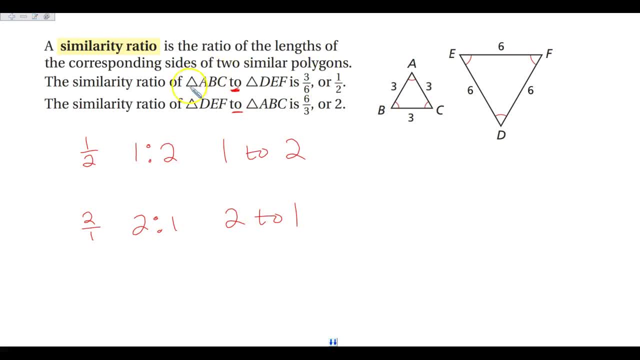 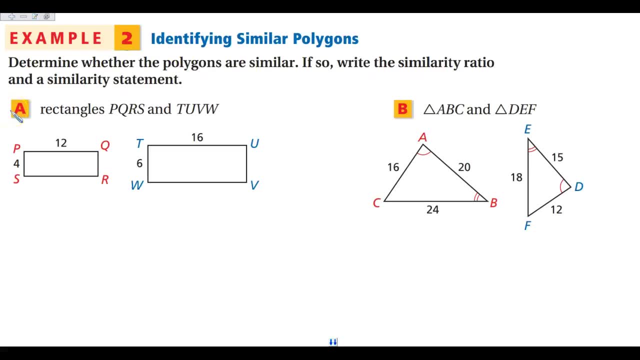 But again, so you make sure you're paying attention to which figure you're doing first, because that will make a difference in your ratio. All right, so let's take a look at example two here, And I want to determine whether or not these polygons are similar. All right, so I'm going. 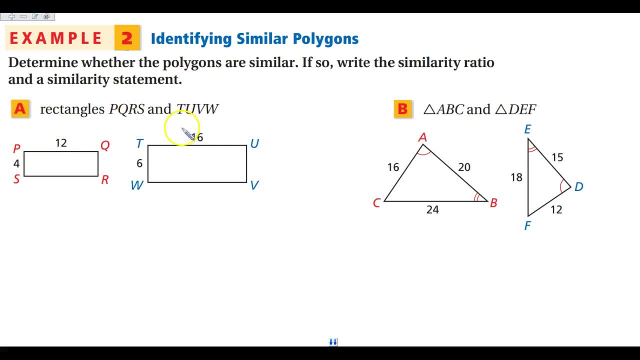 to look here at A. I have rectangles, PQRS and TUVW. First things first is we need to pull all that information that we did in chapter six with our knowledge base about what do we know about rectangles. Well, we know in the definition of a rectangle that it has four right angles. 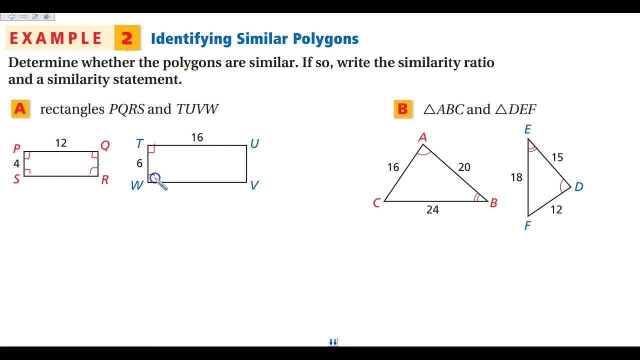 All right, so I'm going to go ahead and label these as four right angles. All right, we also know that a rectangle is still a parallelogram, So opposite sides are congruent. So if PQ is 12, then SR is 12.. If PS is four, then QR is also four. All right, if TW is six. 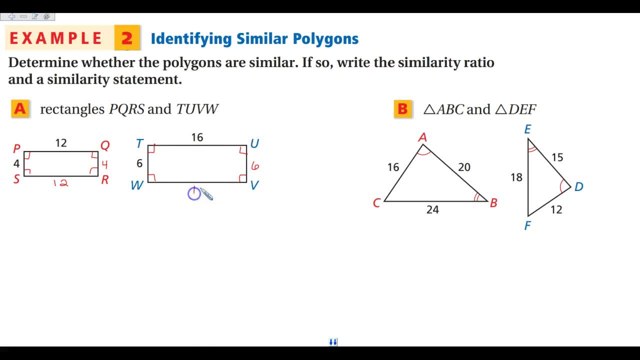 then UV is six, And if TU is 16, WV is also 16.. So now to determine whether or not our figures are similar, we need to hit two checkboxes. we need to have all the pairs of angles are congruent. So when I look here, all these pairs of angles are going to be congruent to all. 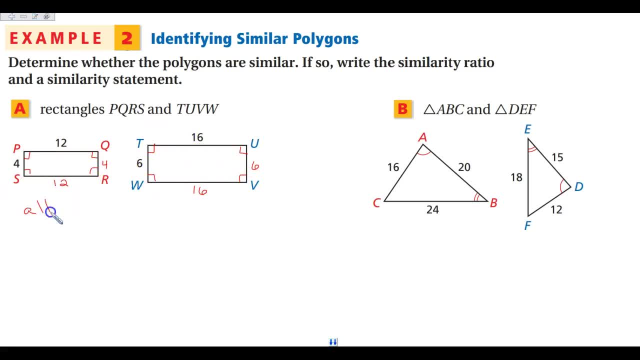 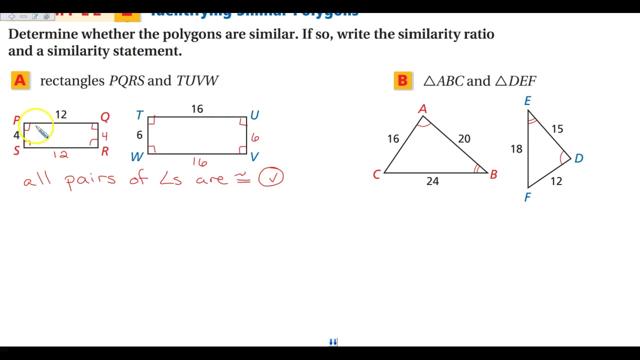 these pairs of angles because they're all right angles, So we know that all the pairs of angles are congruent. So that's like a checkbox for us right there. We needed to know that. Okay, the next thing that we want to do is determine whether or not the sides are proportional. So 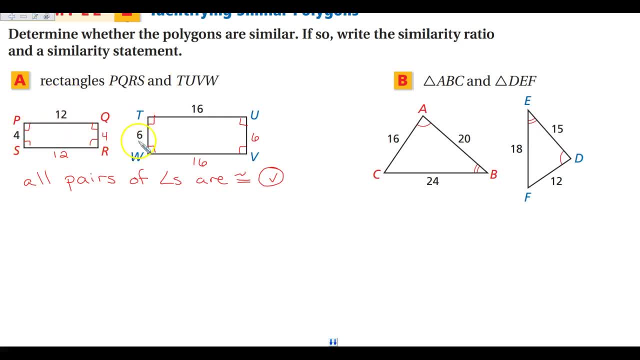 what I'm going to do. because opposite sides are proportional, I'm going to hit two checkboxes. So if the opposite sides are congruent here, I only have to do two pairs of sides. So I'm going to do four, which is PS. Now the side that's going to correspond with PS is going to be TW over here. 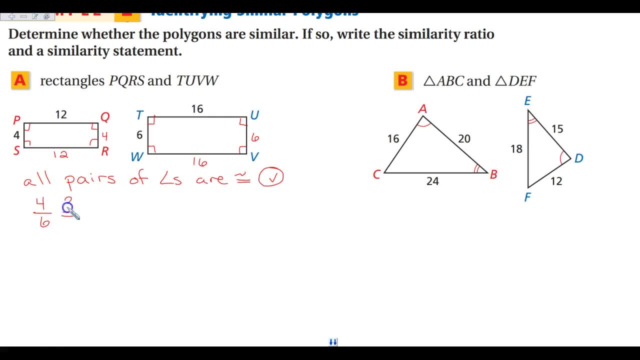 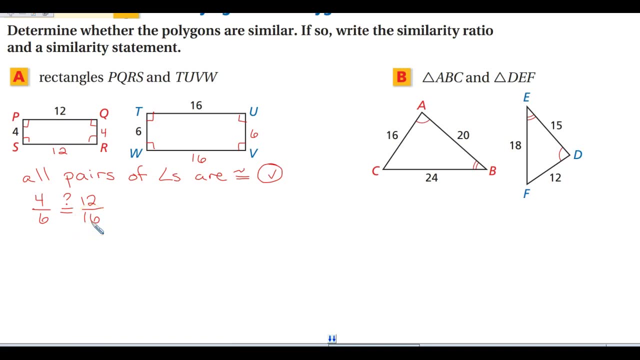 so be four over six, And I want to know whether or not that equals my longer sides, which is going to be 12 for my smaller figure and 16 for my larger figure. Again, notice that I did smaller figure on top, larger figure on the bottom. Okay, so now what we're going to do is we are 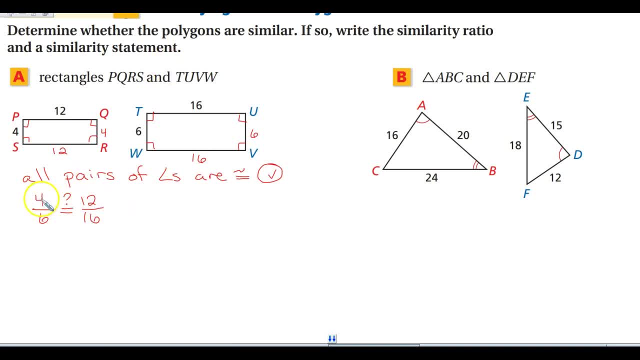 going to reduce both of these fractions. So four over six is going to reduce to two-thirds And 12 over 16 is going to reduce to three-fourths. These are not equal. So because these are not equal, that means that my rectangles are not going to be similar. So we can say that PQRS. 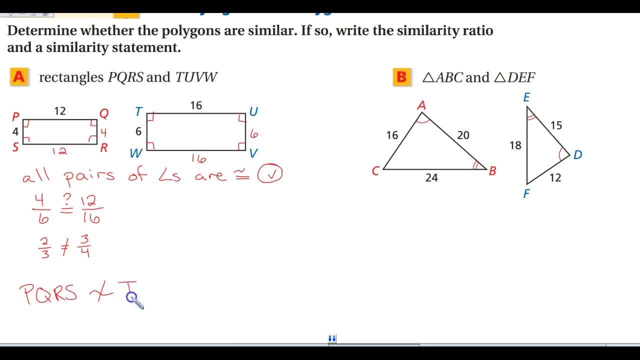 is not similar to TUVW, All right. so again, they're not going to be the same. So we're going to, because, even though all the angles are congruent, their sides are not proportional. So we're going to go over here now and take a look at part B With B. I'm going to start off by doing the same thing. 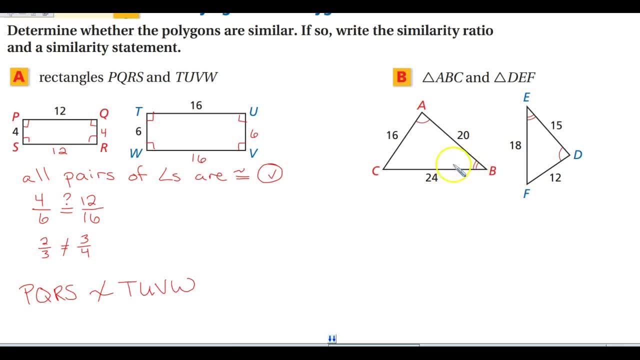 that we did before. as I'm going to start by looking at my angle measures. Okay, I know that angle A is congruent to angle D, because those are marked. I know that angle B is going to be congruent to angle C And I know that angle C will be congruent to angle F. Now why do I know? 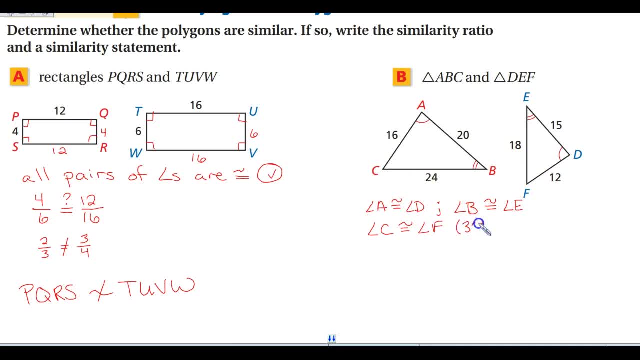 that C and F are congruent. Again, that is my third angles theorem. That is how I know, because I know that two pairs of angles are marked congruent, So that means that the third pair must also be congruent, So I know that all of my angles are congruent. That is a check mark that I 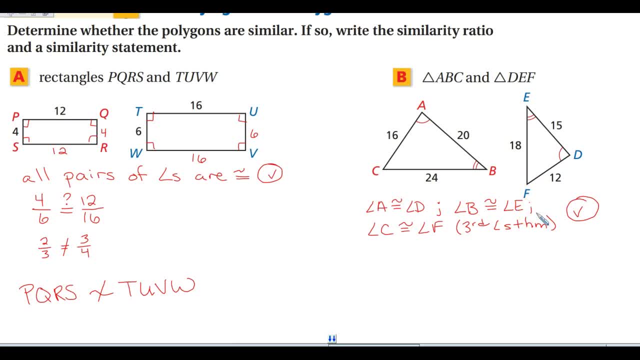 need. So the next thing that I'm going to do is determine whether all of my sides are going to be proportional. So I'm going to start by again, like we did in the last example, we're going to look at labeling our sides as small, medium and large so I can put them in the right ratios. So in this, 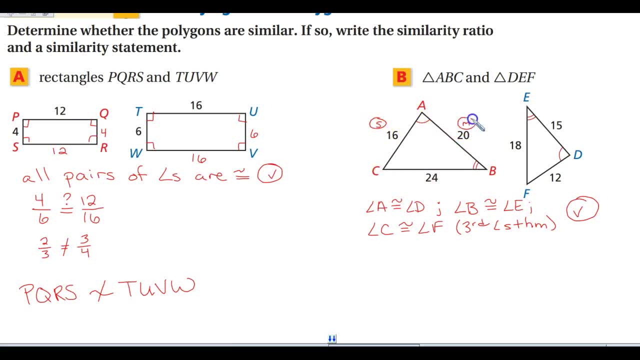 triangle: 16 is my smallest side, 20 is the next longest, and then 24 is my longest side. Same thing over here: 12 is my smallest side, 15 is my longest side and then 24 is my longest side. 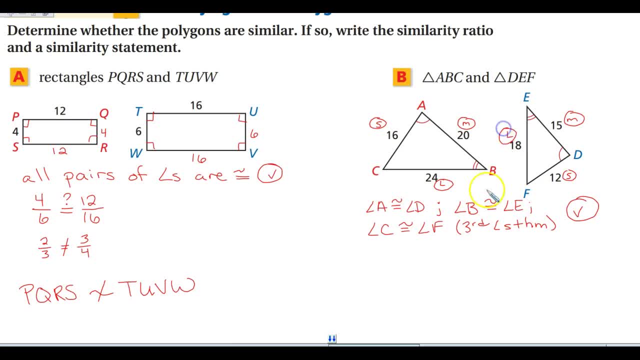 So I'm going to start by again, like we did in the last example, we're going to look at labeling our sides as small, medium and large so I can put them in the right ratios. So I'm going to start by: 17 is my medium length side and 18 is my long side. So what I'm going to do is I'm going to put my left. 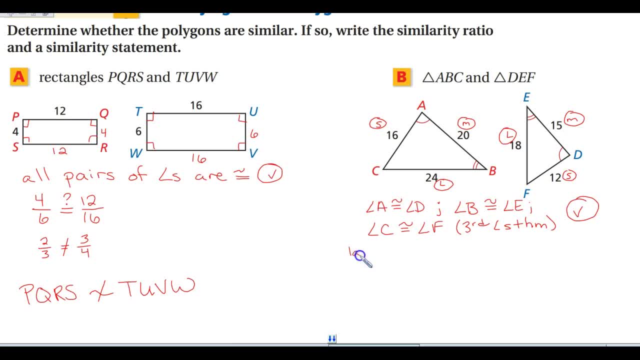 triangle over the right triangle. So everything that I'm going to do here is I'm going to set up my larger triangle over my smaller triangle, And I'm going to do this to help keep me organized. All right, again, it doesn't always have to be small in the numerator, So my smallest side for 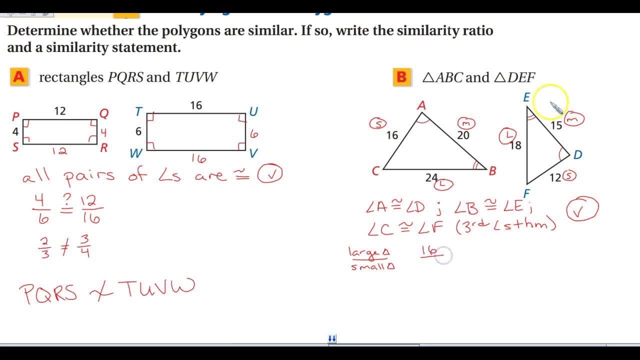 my large triangle is 16.. My smallest side for my smaller triangle is 16.. And I'm going to set up my smaller triangle is 12.. I want to know whether or not that is going to equal my medium side, which is 20, over my medium side, which is 15.. And I want to know: does that equal my longest sides of? 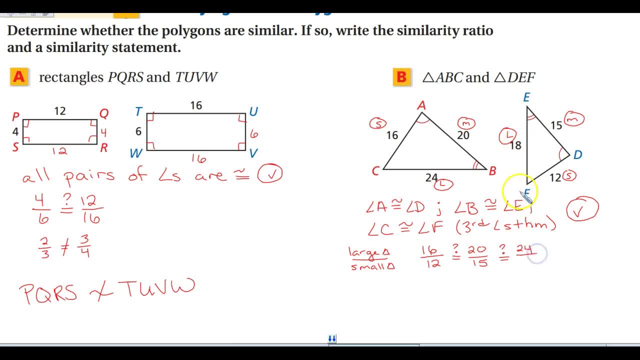 my biggest one, which is 24, over my smallest one, which is 18.. So every single one of these fractions has the larger triangle in the numerator, the smaller triangle in the denominator. All right, so 16, over 20 is going to reduce to four thirds. 20 over 15 is going to reduce to four thirds. 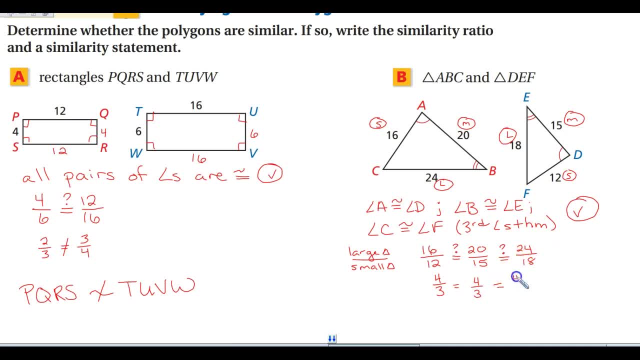 And 24 over 18 is also going to reduce to four thirds. So, because they all reduce to four thirds, four thirds is going to be my similarity ratio, Since all of the sides are proportional, all of the angles are the same measure, My triangles are going to be similar, And four 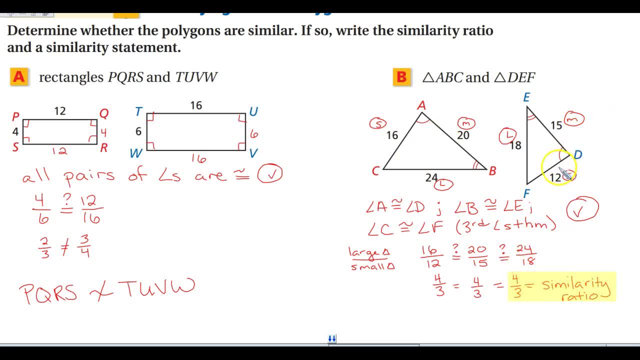 thirds is going to be my similarity ratio, from my large triangle to my small triangle. Okay, if you did it the other way around, three fourths would have been your similarity ratio, And that would be fine, Because it doesn't tell you in this problem which way to write your similarity ratio. 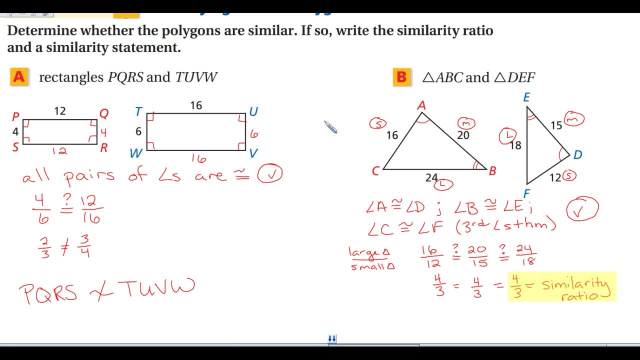 whether you're writing large to small or small to large. either way is fine, Because, again, it does not specify. All right, the next thing that we need to do, because we wrote our similarity ratio, is then we need to write a similarity statement. So our similarity statement is just like our congruent statements. 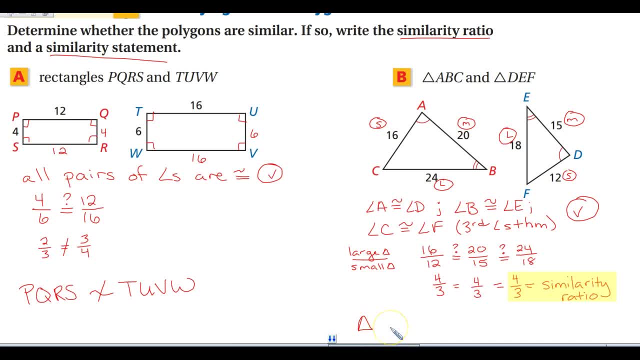 We have to match our angles, We have to make sure our sides are corresponding, But instead of our congruent symbol, we are writing our similarity symbol. So I'm going to start with triangle ABC And it is going to be similar to triangle. Now angle A is going to match with angle D. 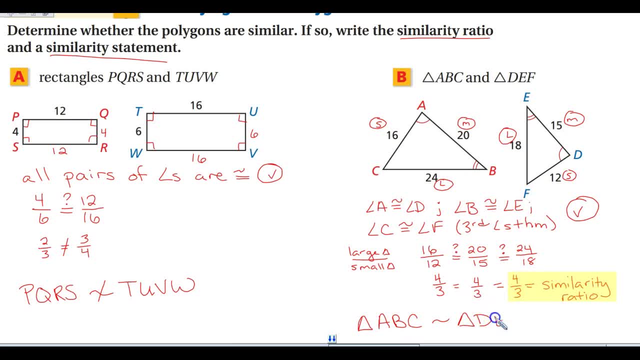 Angle B is going to match with angle E And angle C is going to match with angle F, So ABC is similar to triangle DEF. So again, in order to prove similarity, you have to have all of your pairs of angles are congruent and all of your pairs of sides are proportional. All right, so if you have any questions on that, go ahead and write them down on your papers now. 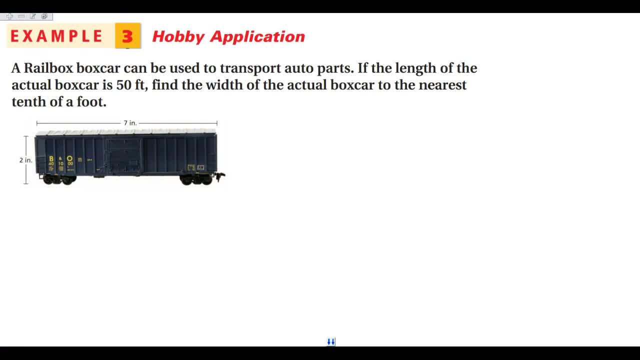 All right, let's go ahead and look at example three. All right, so with example three we have a rail box car, so a train car can be used to transport auto parts If the length of the actual box car is 50 feet. we want to find the width of the actual box car to the nearest tenth of a foot. 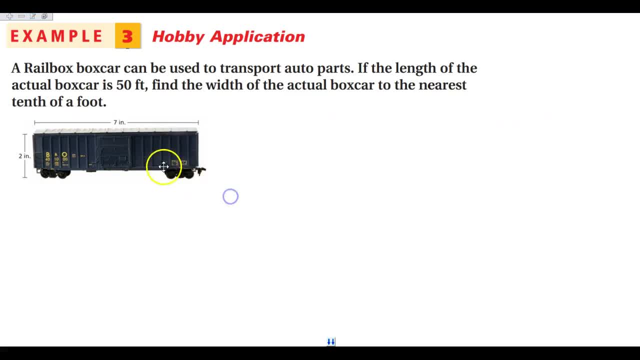 So what we're going to do here. I'm actually going to kind of shrink this up a little bit to make it look like it's going to be a model, And I'm going to copy and paste it. So what you may want to do. 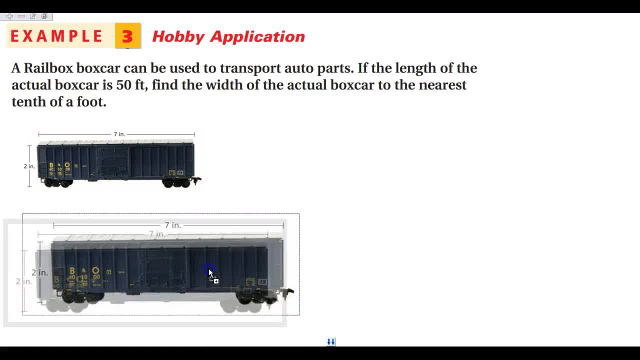 is just sketch, like another rectangle on your paper, so you can kind of see what we're looking at. All right, so this won't be seven inches and this won't be two inches. All right, so what we have here is the length of our box car. The model is seven inches, so I'm going to write: L is equal. 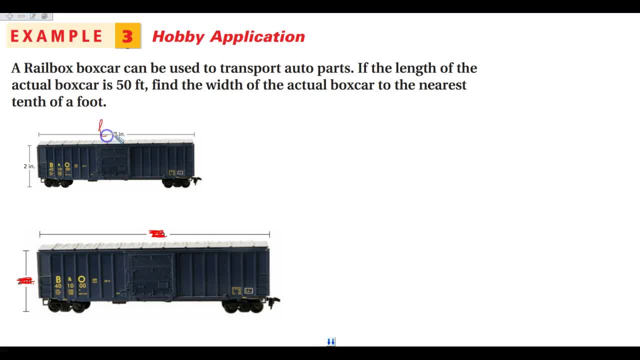 to seven inches. My L's are getting wonky. There we go. Okay, that's going to make my width two inches, All right. so the length of the actual box car is 50 feet and the width is what we're looking for. 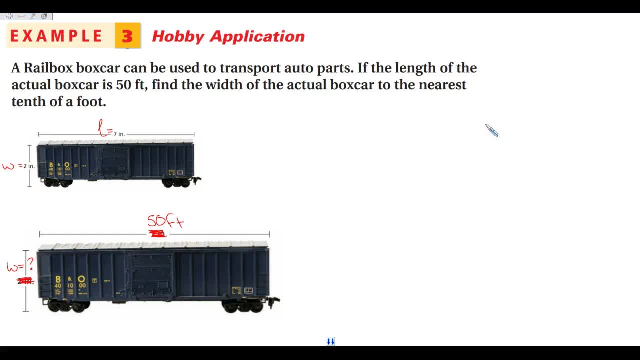 Okay. so when you do a model, okay. so right here we have a model of the box car- When you do a model, it will always be similar to the actual size. okay, to the actual figure. So I know that this box car is going to be similar to the real thing. So what I'm going to set up? 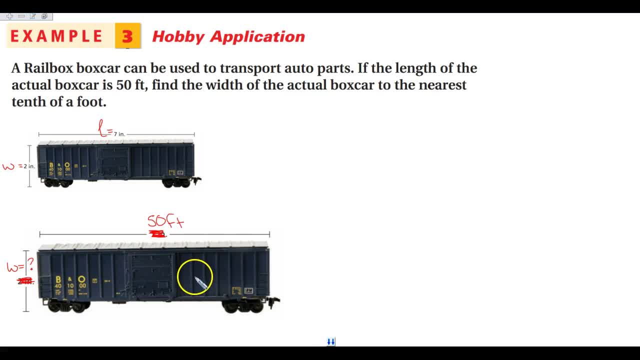 here is: I'm going to set up a proportion where I'm going to put the model over the actual figure, So I'm going to do the smaller one to the larger one, All right. so the width or the length of my smaller figure is seven inches. 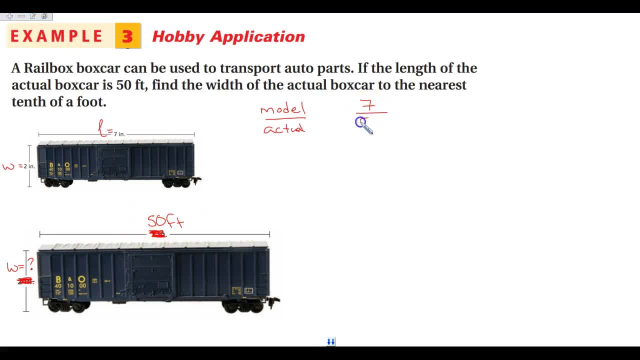 The length of my larger figure is 50 feet. I don't have to worry about units here, because I'm going to go. this is inches, inches. This will be feet, feet. It will be fine. You don't have to convert anything, It's fine, All right. the width of my model box car is two inches.